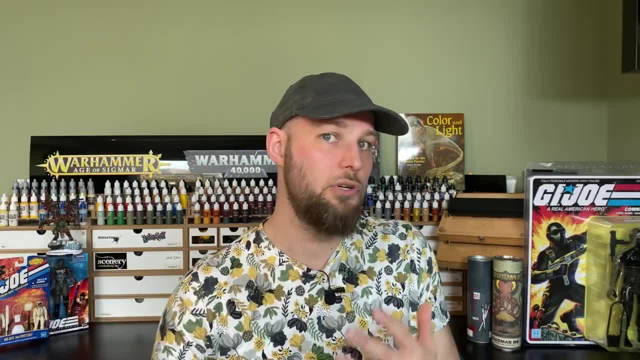 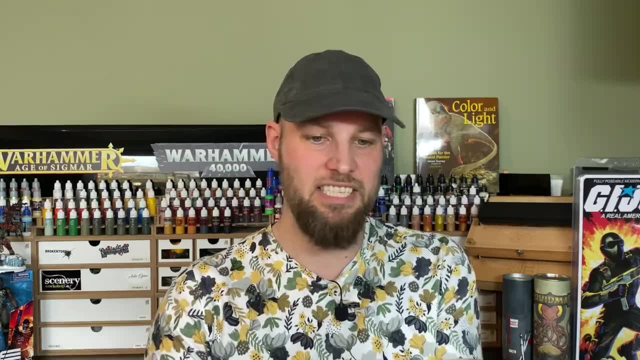 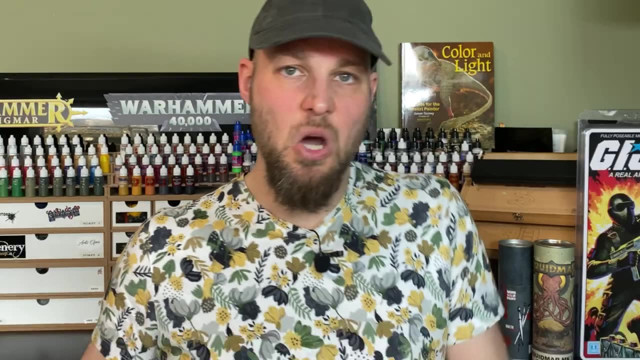 It's miracle stuff. It really is miracle stuff. I'm going to compare practicality and that's just my experience, What I encounter. How is it packed? How's the mixing? Is it sticky or not? Stuff like that- Things you come across while using it. I'm ready Work life, AKA curing time. How long does it? 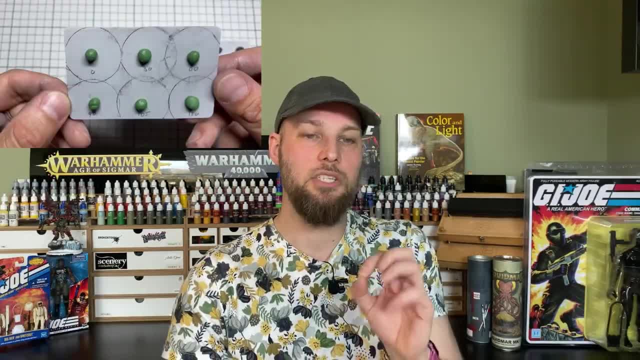 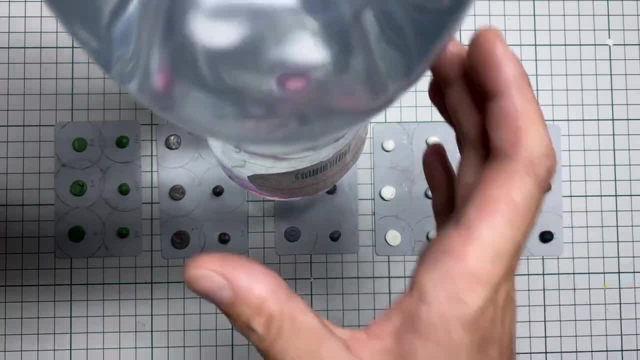 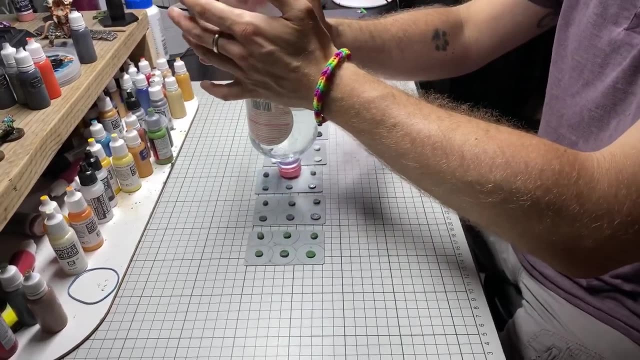 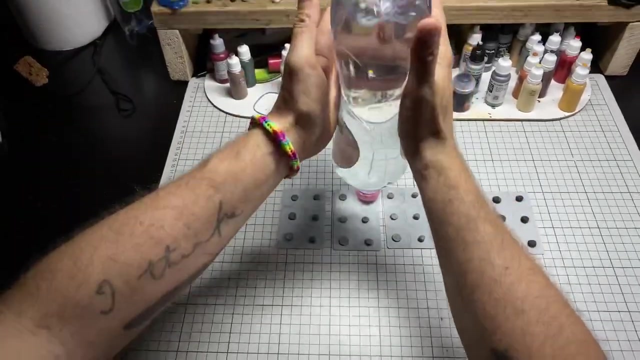 take to cure, And I'm going to do this by making small balls. I'm going to do this by making small balls and trying to flatten them using a water bottle of approximately one kilogram, or about two pounds for some of you, And I'll be doing that at 0,, 30,, 60,, 90,, 105 and 120 minutes after. 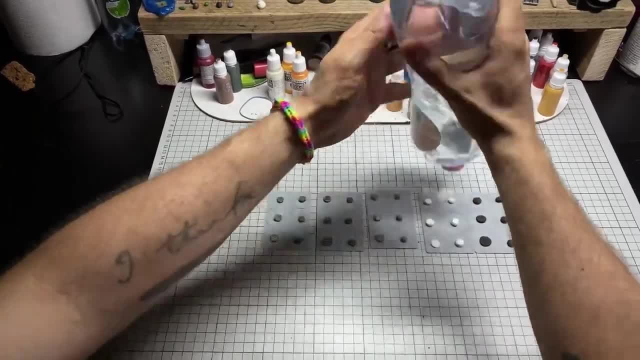 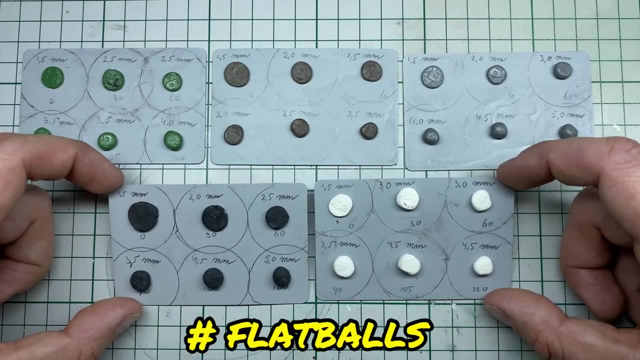 mixing So you get a nice overview of, well, how long it takes for them to cure And I measure how flat the balls get- Hashtag flat balls, I guess. So that would give us an indication of how malleable the stuff is over time. Science- 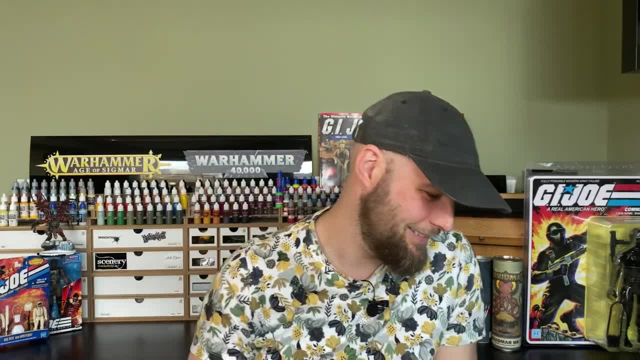 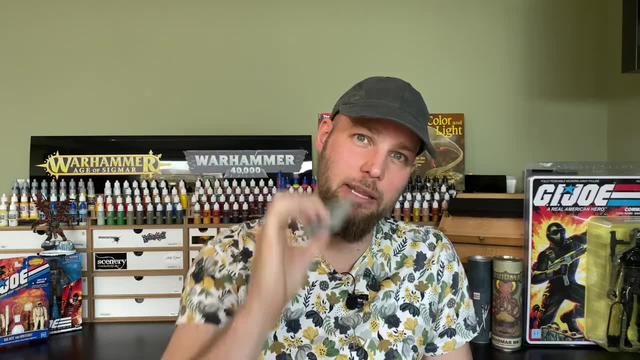 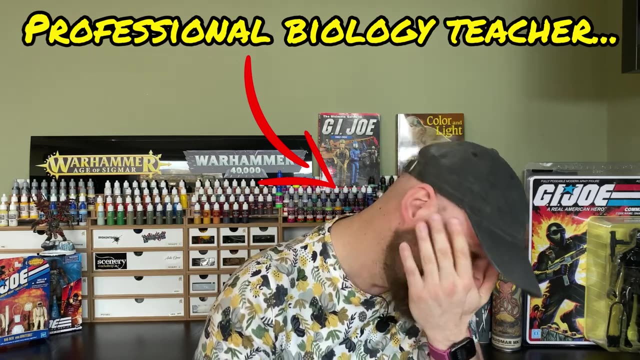 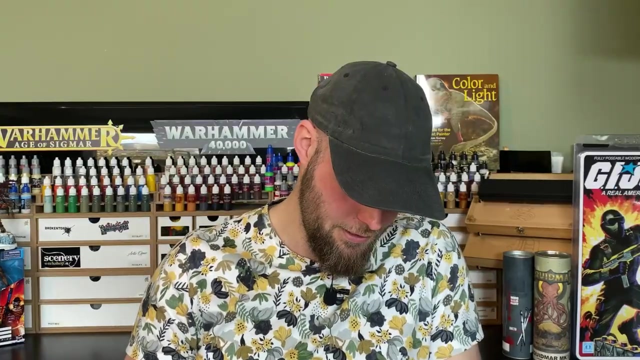 So I measured all flattened balls. I really have to come up with something else for that. So I measured the height of my tiny balls. What's a different word for balls? Let me Google balls synonym. I'm not going to say that in my 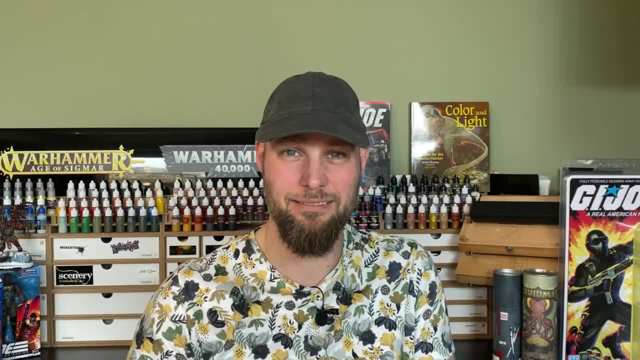 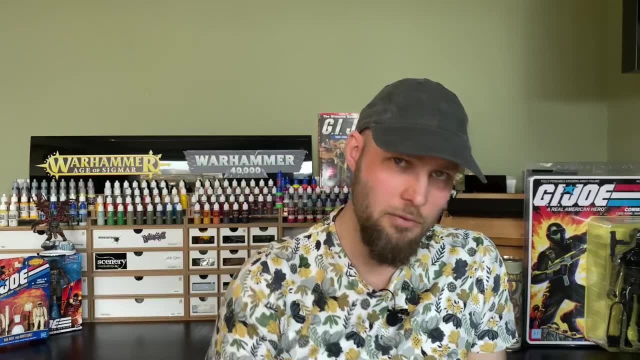 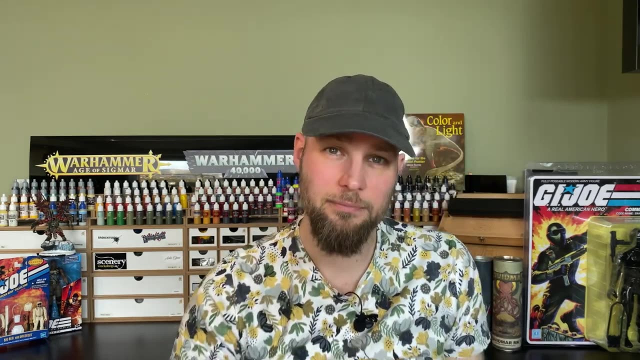 YouTube video. Let's just call it balls. Okay, By measuring the height of the balls, I could get a clear indication of how malleable the stuff is over time. All of the products are very malleable for about 30 minutes and then they start to differ. So if you look at the graph- this graph- 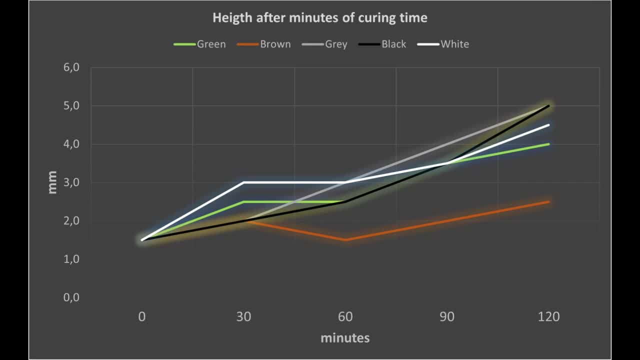 you see that compared to the other products, brown stuff stays soft for a very long time And even after the claimed work life of 90 minutes it's still very malleable. Green stuff cures slowly but steadily, But of all of the stuffs, gray stuff cures the fastest, Both black and white milliput. 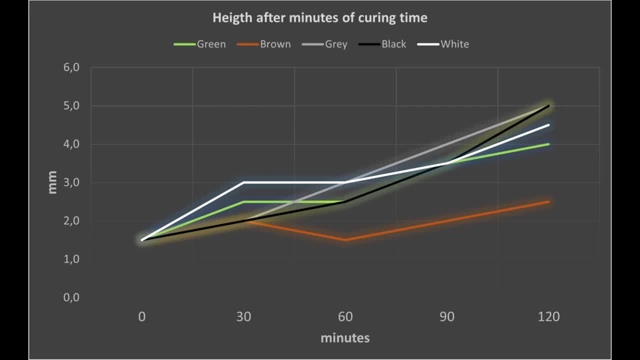 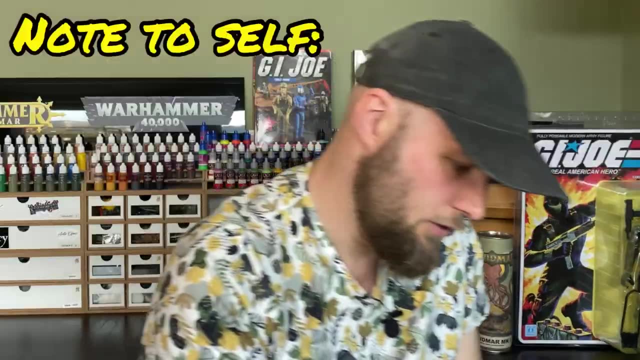 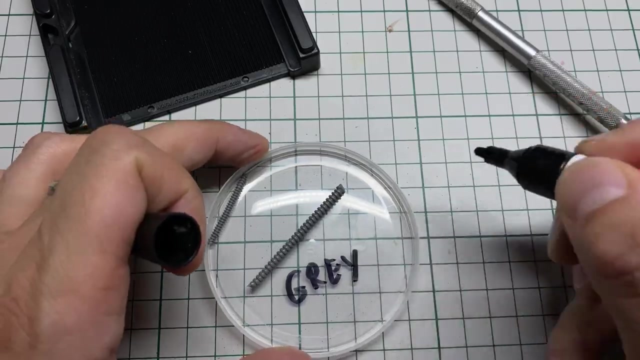 take a little less time to cure than green stuff. And now for something completely different: Flexibility. Don't ever do that again. To test flexibility, I will use a green stuff world's roll maker to make rolls. That's basically what a roll maker does, isn't it? 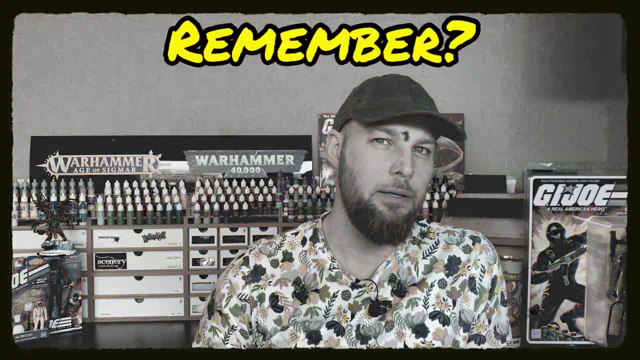 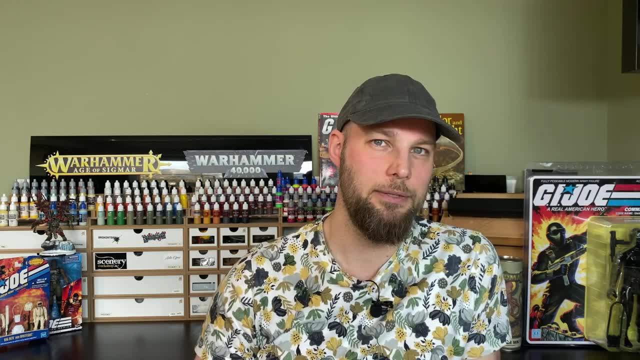 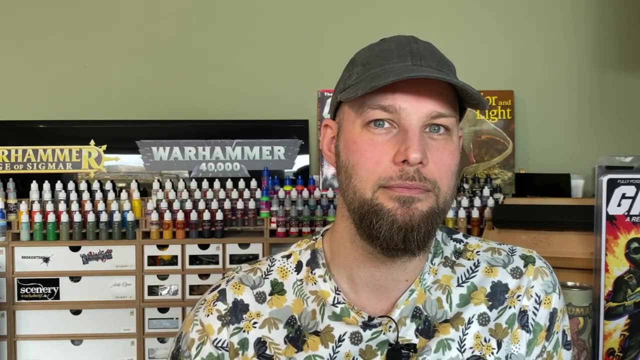 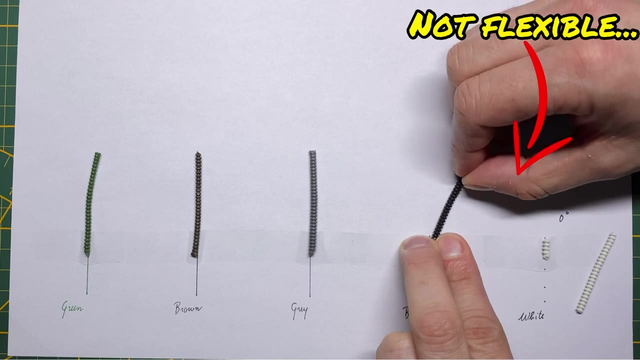 And I let them cure for about five months Thoroughly, While in reality 24 hours would suffice. Yeah, let's say, something came up. I'm a bit of a procrastinator sometimes. I then taped the rolls to a piece of paper and I started bending them And I measured the angle at which the roll would break. 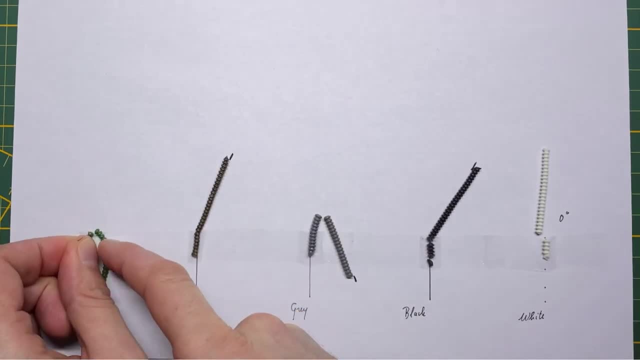 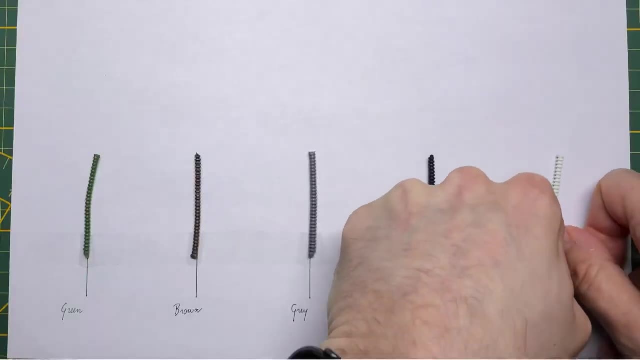 The greater the angle, the more flexible the product is. Easy Science, And that's where the real difference is showing. I wasn't even able to bend the white stuff at all. It immediately broke when I taped it down. So that's zero degrees Brown stuff, although it cures. 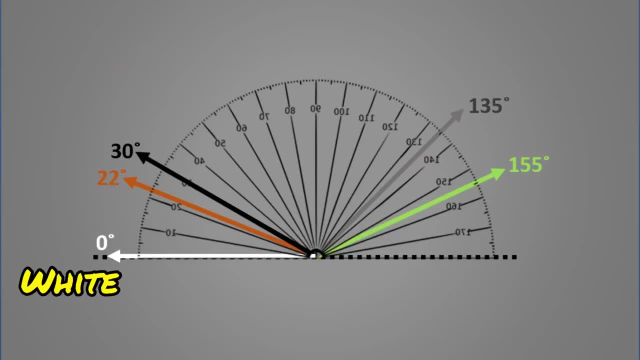 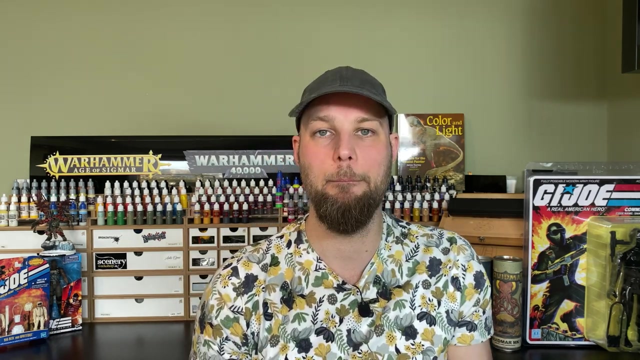 very, very slowly it gets pretty hard. I could bend it 22 degrees, which makes it of all the stuffs- the green stuff, brown stuff and gray stuff- the least flexible. After that we got the black milliput with 30 degrees and then a big gap, A very big gap. Look at those differences, I mean. 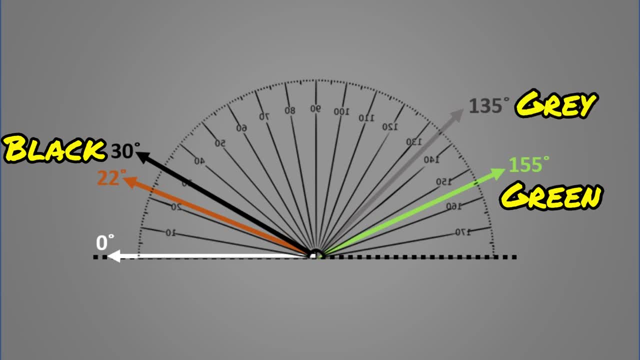 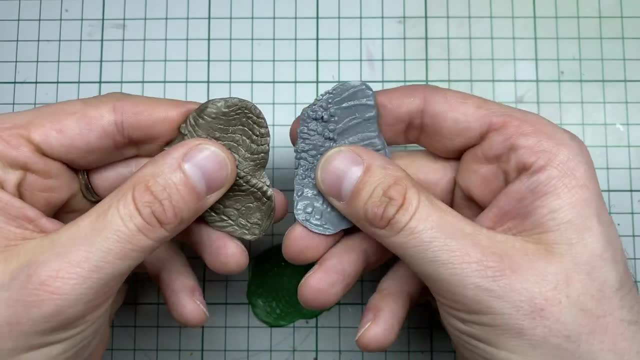 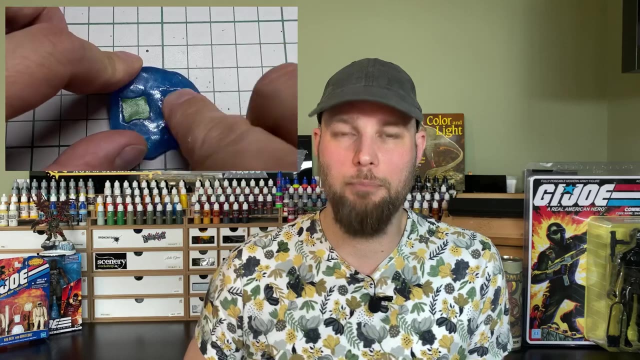 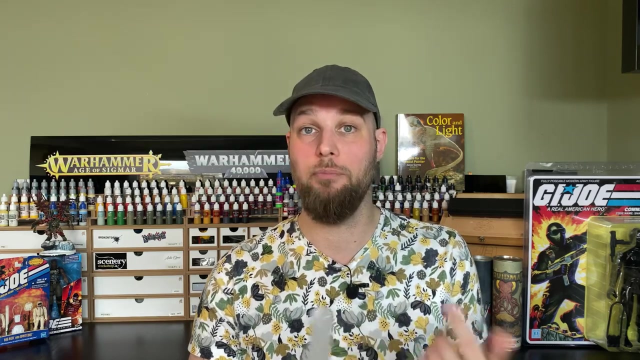 green stuff is the most flexible. Gray stuff is a bit less flexible than that, but still green stuff and gray stuff are both pretty flexible. Using blue stuff, I made some simple push molds and I used a textured roller pin to make some Warhammer bases. to check the ability to obtain details, 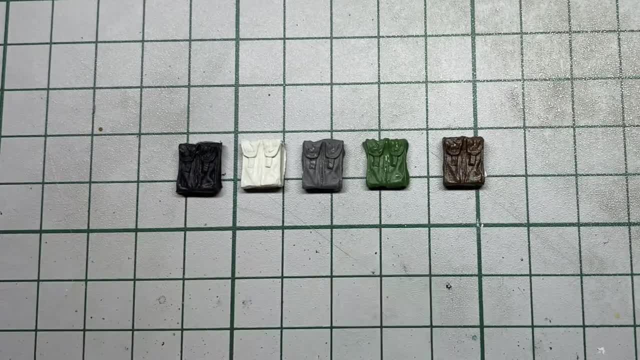 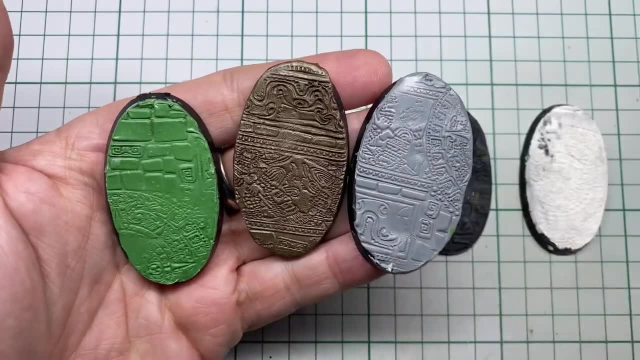 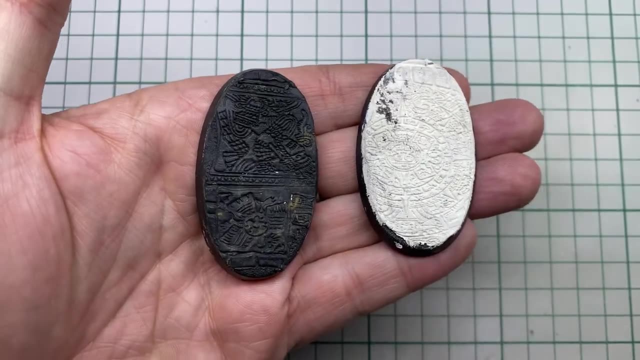 If we compare all these copied details we don't really notice a difference, And also the different bases I made with the roller pins seem to look quite similar in quality Due to the stickiness and the fact that it's quite brittle. the ones made with milliput look a bit more. 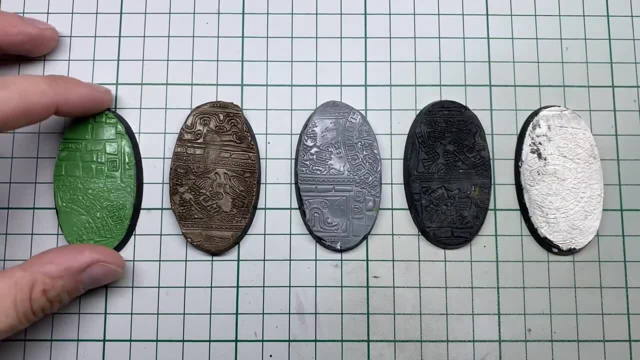 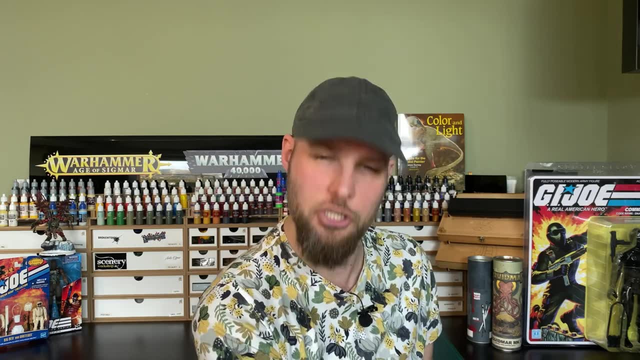 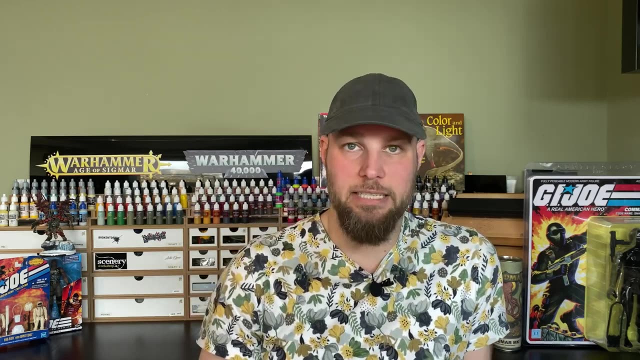 damaged, But that could also be a look you desire, of course. They all sculpt quite well, They're very, they're, yeah, they do what they should do And that's a good thing. One more thing And last practicality, which is just my experience using 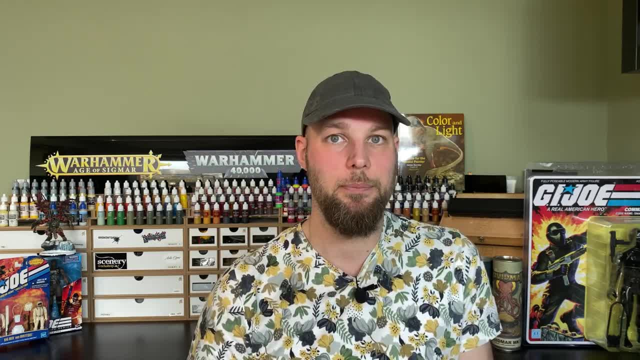 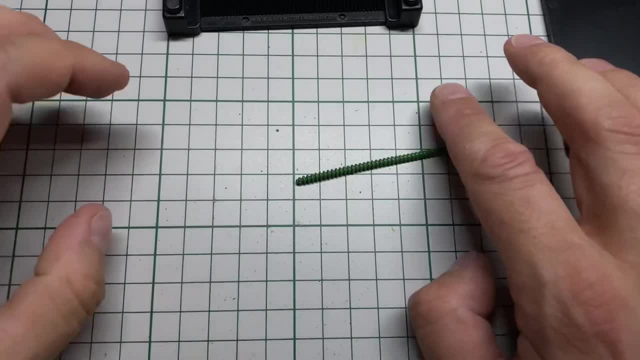 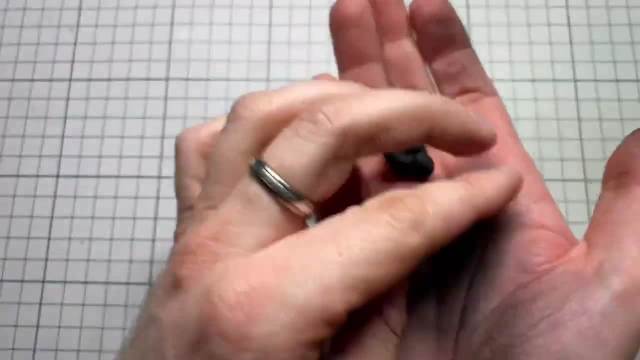 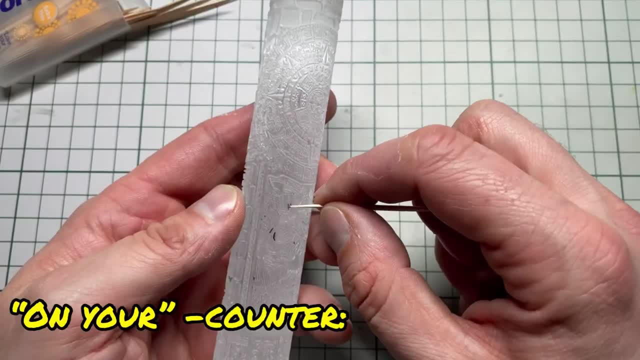 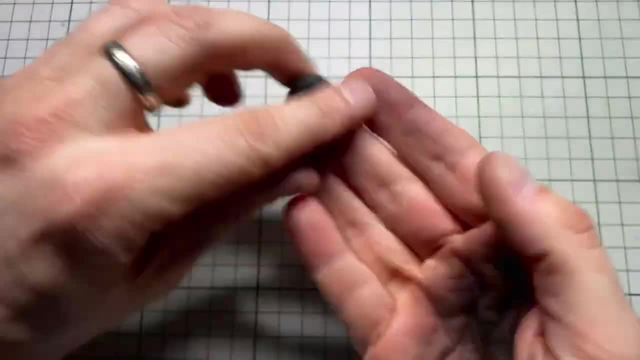 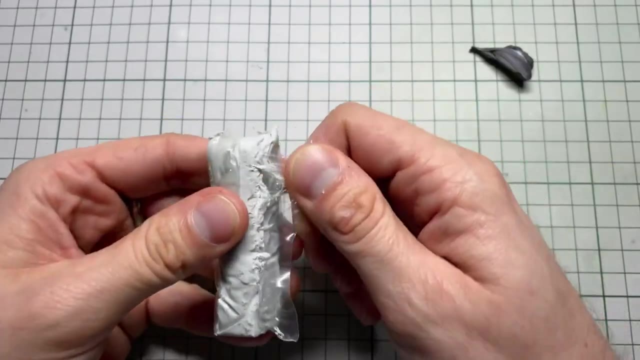 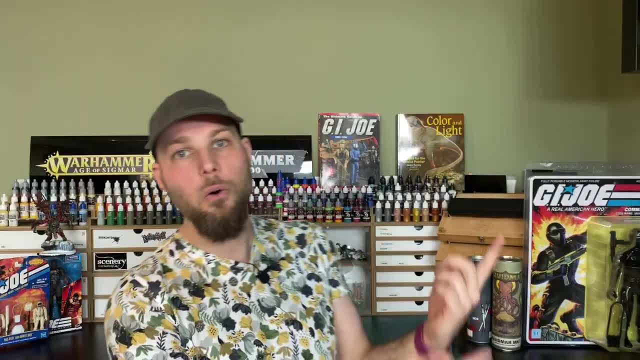 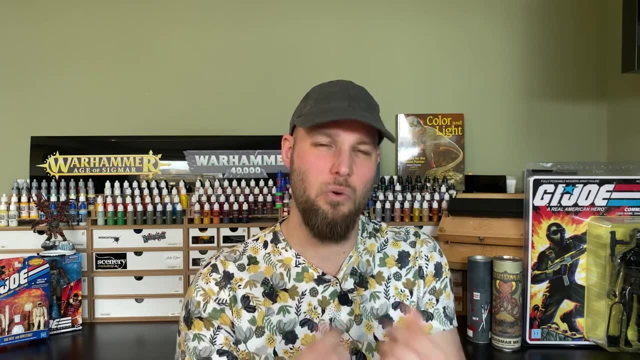 away the plastic that it was wrapped in, So I could throw away this, which is quite a waste. Then the mixing It is. it's it's very hard already, So I literally got blisters on my hand. Perhaps I had an old. 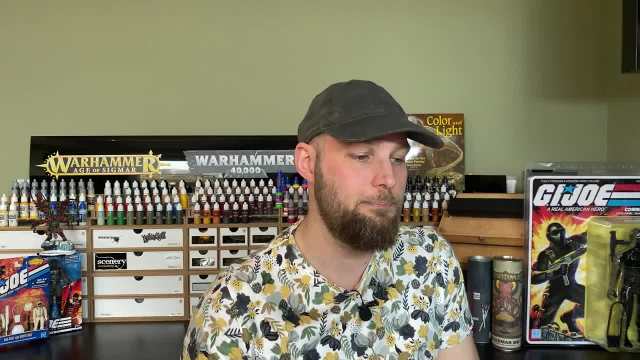 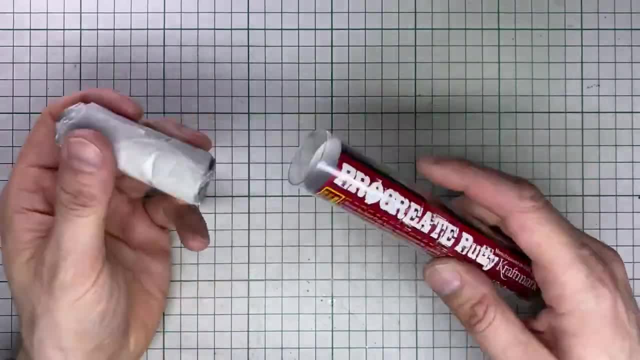 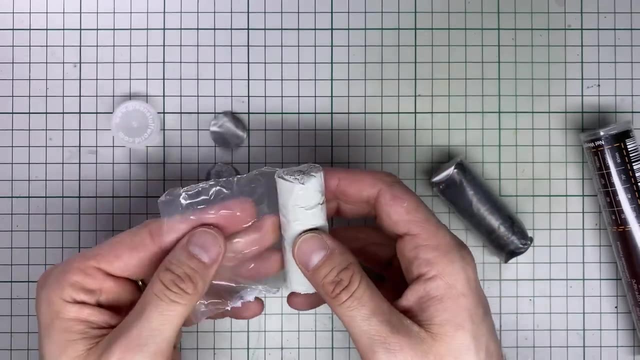 batch. I don't know what idea I like working with it, but I did order another batch, 16 paranoia filled days later. So after a few weeks I received my fresh gray stuff And the first thing that strikes me is that the packaging differs from the batch that I used in my experiments. The wrapping is tougher. 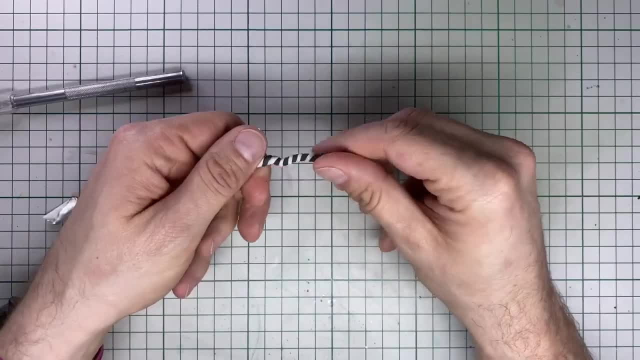 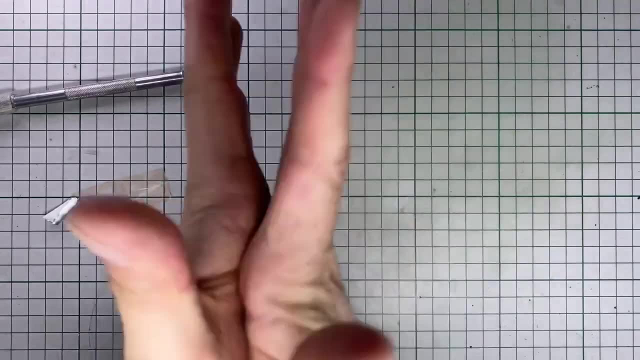 and the putty seems to stick less to it. It is still quite hard to mix, though, but not as hard as my old supply was. All in all, I guess my suffering was mostly influenced by the shelf life of my old supply of gray stuff. And now back to the video. 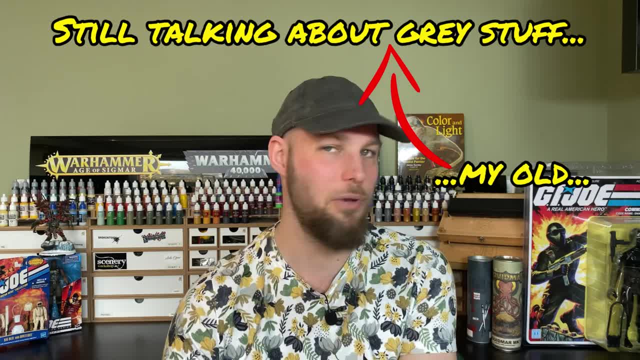 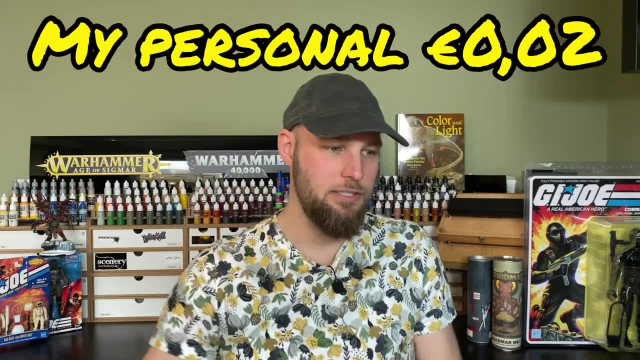 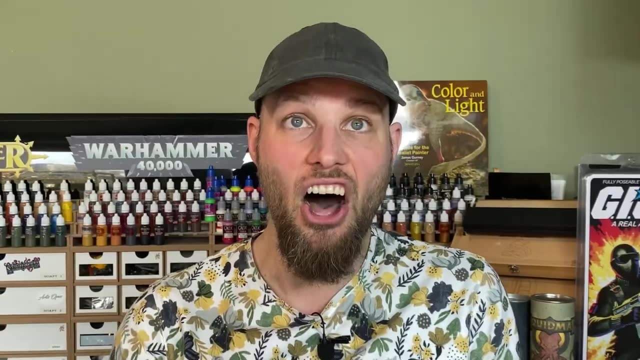 Meanwhile, back in the lowlands. I like working with it. I don't like working with it, but I like the end result of gray stuff. So my recommendations- because what is the answer? Which one is the best? That depends what you want to do with it. I like using green stuff to fill gaps. 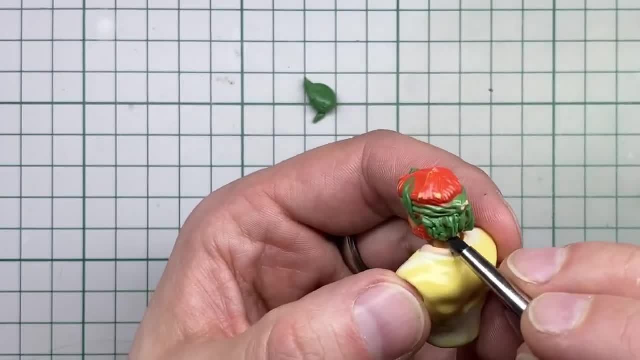 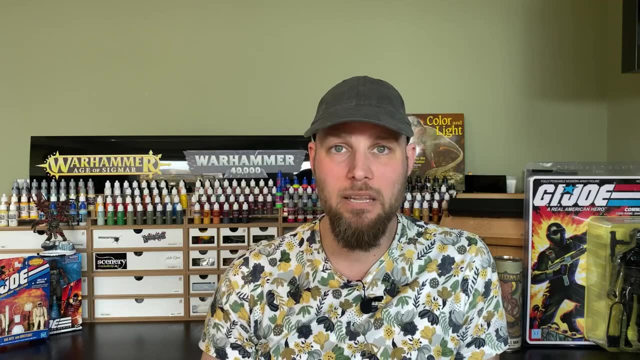 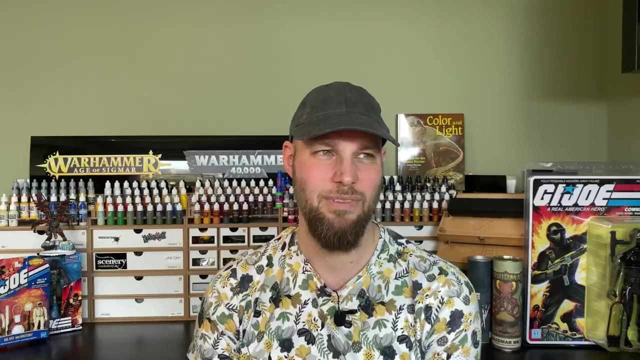 My miniatures and I like green stuff to sculpt hair and beards. But for that I like brown stuff even more because it has a longer working life. Milliput, black and white, I don't use. I don't use that a lot anymore. I don't like it. That's it For making details for. 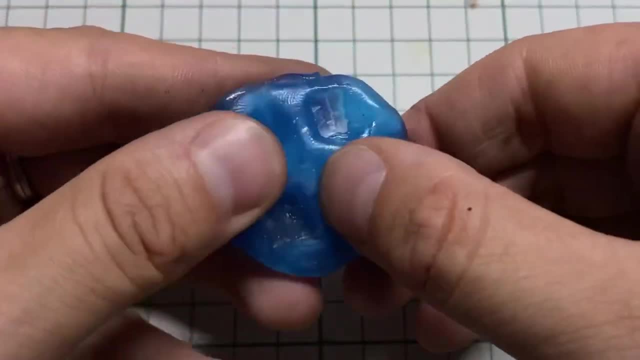 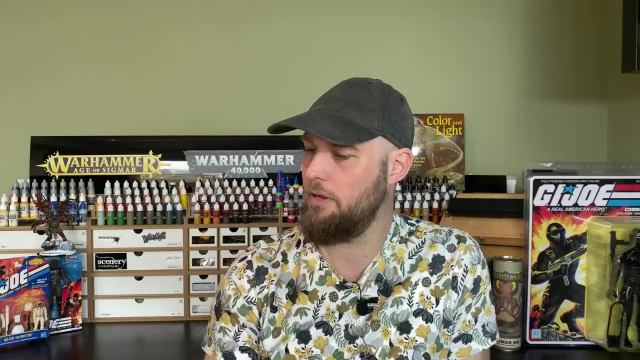 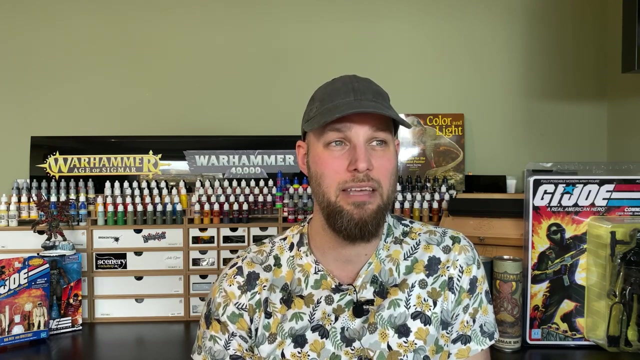 my GI Joe's using blue stuff. It's excellent And it's a bit cheaper than the other products. Gray stuff I have very ambivalent. It's hard work mixing it And you've got a lot of ways. but in the end, when I want to make my 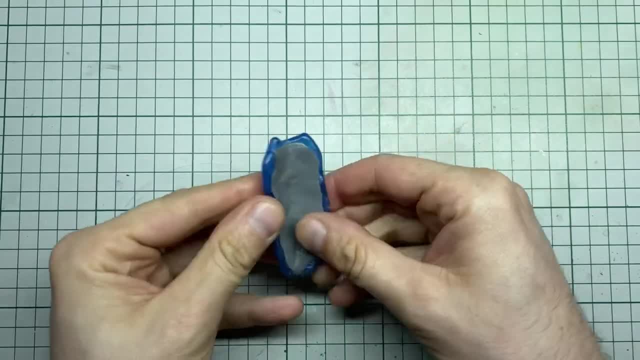 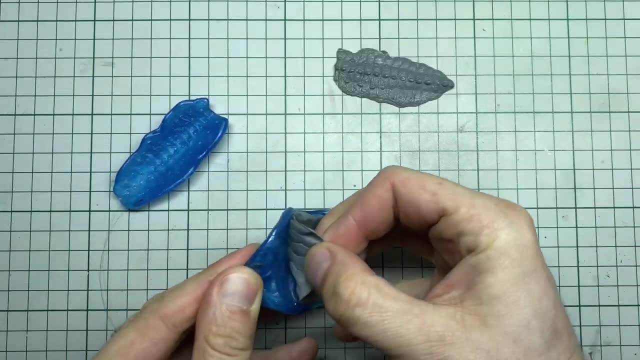 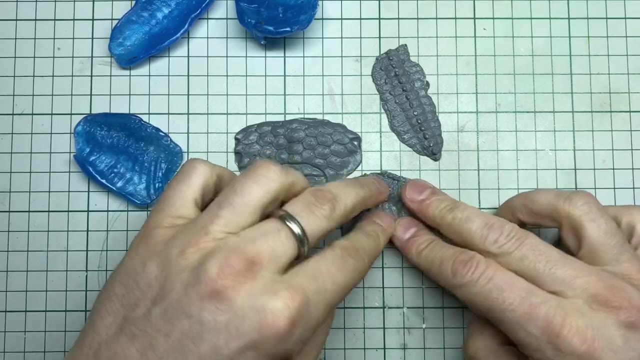 Warhammer bases fast. I use grays. After 30 minutes I can remove it from the mold and I can let it cure And I can make another copy. where that's impossible with green stuff, brown stuff or the milliput, You really have to. you really have to let them sit inside the mold for at least. 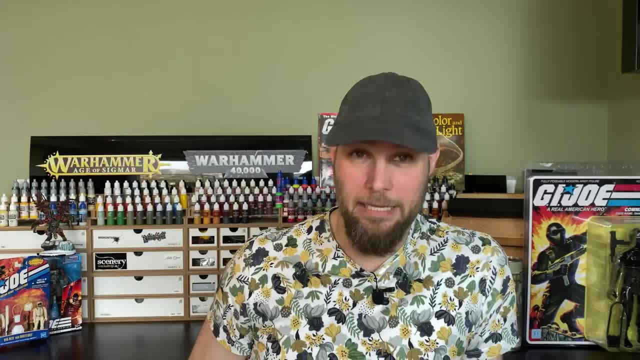 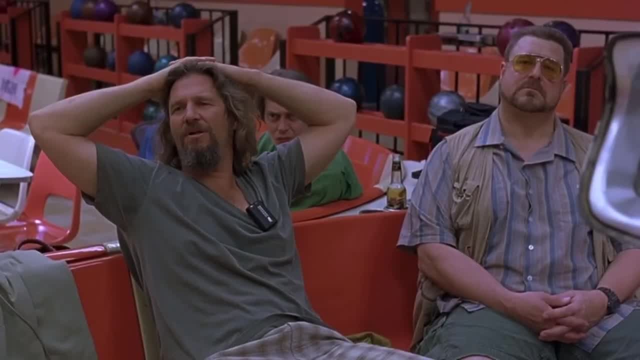 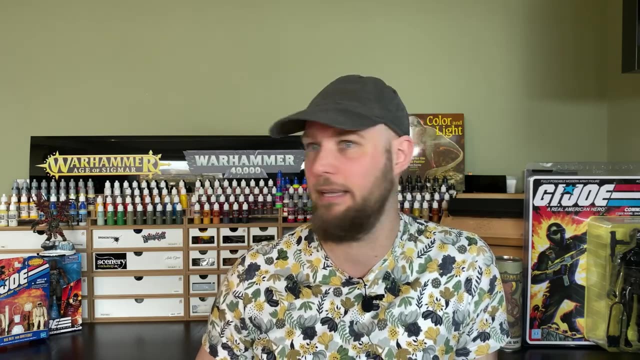 two hours before before Removing it again. which one is the best? All of the stuffs I like, Milliput the least. Yeah Well, you know, that's just like, uh, your opinion, man, It hasn't used it And if you like it. 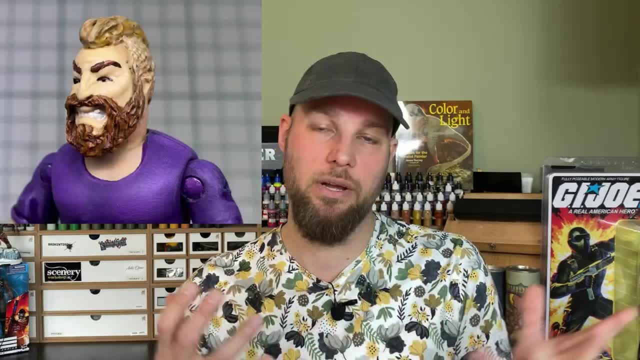 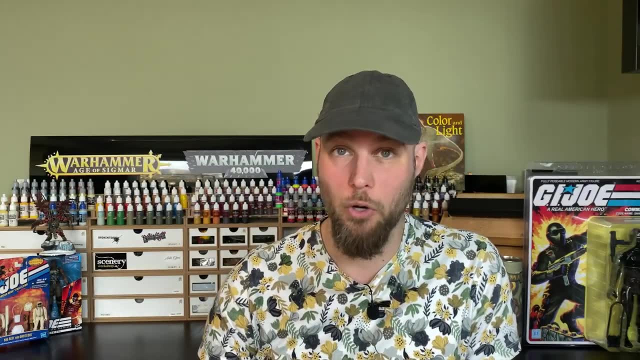 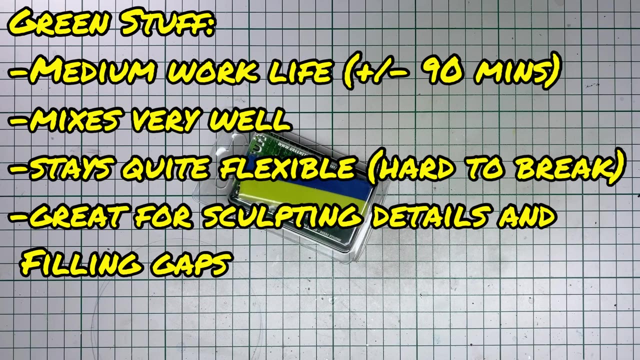 feel free to like it. Whenever I sculpt some beards or I sculpt some hair or I sculpt a mustache, I'm pretty sure I would like to use green stuff or brown stuff. It's alive and kicking. They're just going in circles. 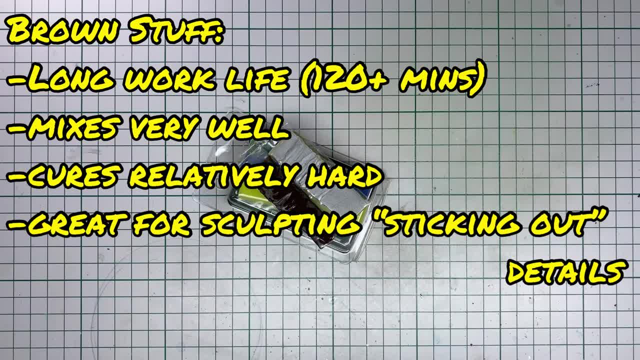 Now you can do whatever you want to them. Yeah, I can do whatever I want. So if you're going to use gray or you can use brown stuff, just use brown stuff, And if you're going to use blue one, you can just use that. 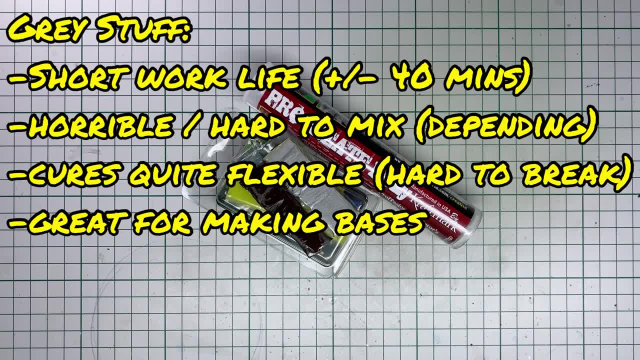 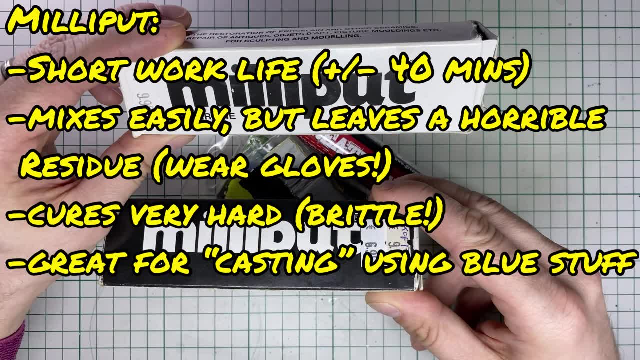 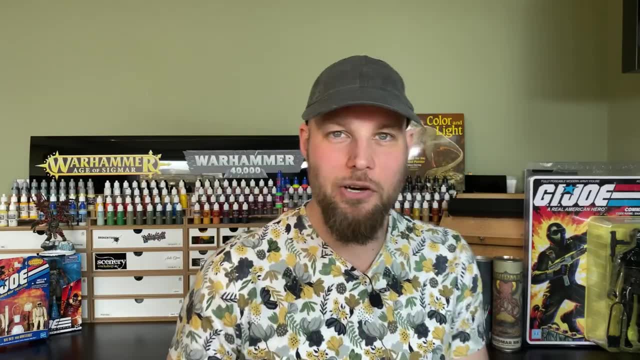 And if you're going to use brown stuff, you can just use brown. It's just, it's just, that's beautiful, Wow, It's like a giant say-so: Yeah, Yeah. and there you have it. now you know which putty you should use for your.